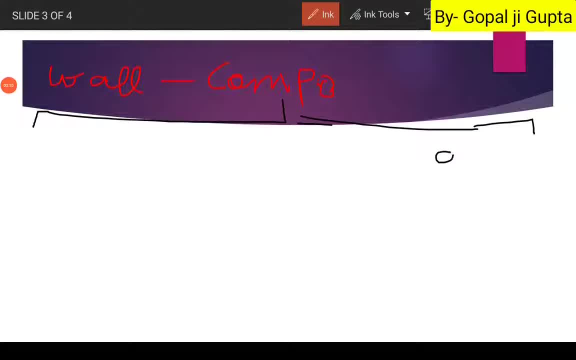 Okay, First group is based on the organic wall. when you have, the organic wall means carbonic, That is, carbon rich, And on the other hand, we have some microfossils which are having minerals in them And, on the other hand, we have some microfossils which are having minerals in them. 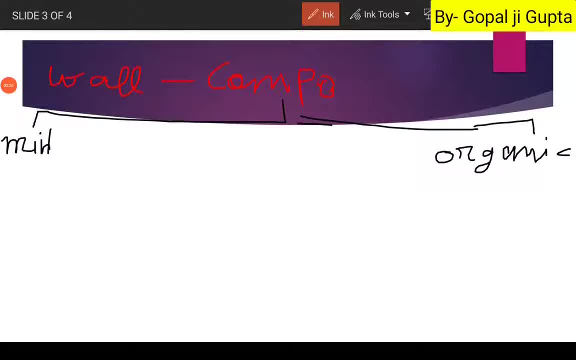 in their world. okay, so now we have classified into two groups: mineral world and organic world. now let's let us see what type of mineral can be there. so the general mineral which we know can be calcite, that is, ca, co3, or we call it a calcareous wall composition. 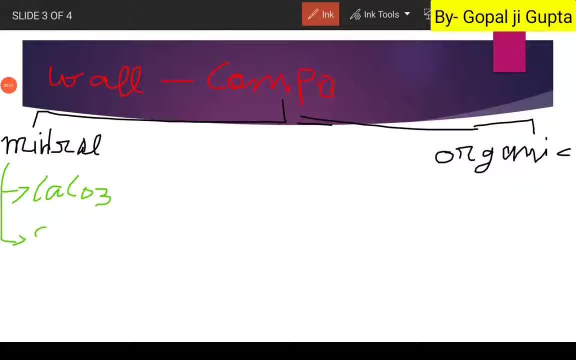 another is si, o2, that is, we call it as a siliceous composition. and the third one is your phosphatic composition- okay, phosphatic. and the fourth and last one is your cytinocalcareous, or the chitinocalcareous, whatever you pronounce it. 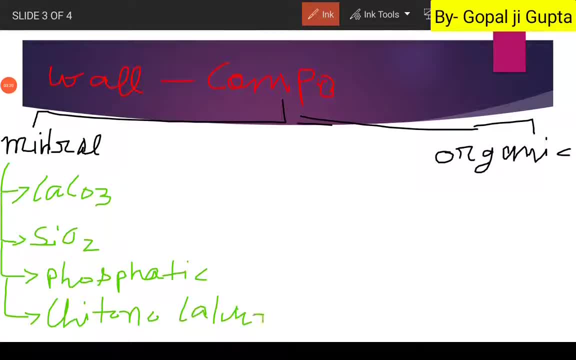 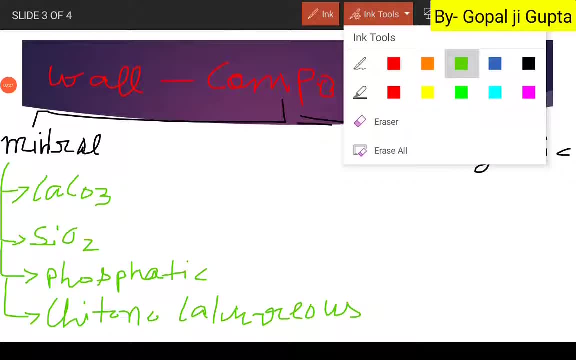 chitino, calcareous. okay, now we will see what minerals are present in these composition. so if we talk about the mineral, the microfossils, having the mineral world of calcium carbonate or the carbonaceous mineral world, microfossils, so we have mainly two. the first one is your. 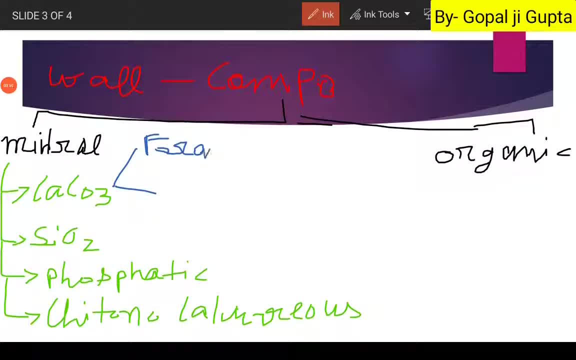 well-known foraminifera. okay, that is foraminifera. oh, it is a little bit glitch in my pen, so another: the calcareous wall microfossil is your nanoplankton. okay, that is nanoplankton. then we will turn towards the si o2 or the siliceous wall composition. 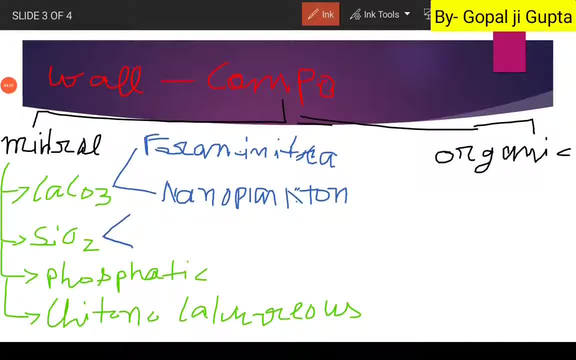 microfossils. so again we have two- i hope you all hear this name- that is radial area- okay, radial area. and other is diatoms- okay. then we have the phosphatic wall composition microfossil that are conodonts- okay, conodonts. then the last one is our cytinocalcareous wall and in this, the mineral. 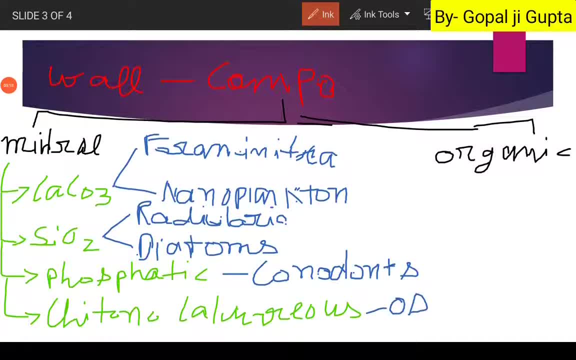 comes are ostracoda or the citinocalcareous wall, and in this the mineral comes, are ostracoda or the ostrogots, OSTRACODS, that is, Ostracodes. so these all are the mineral walled microfossils. there are a lot of other microfossils also. 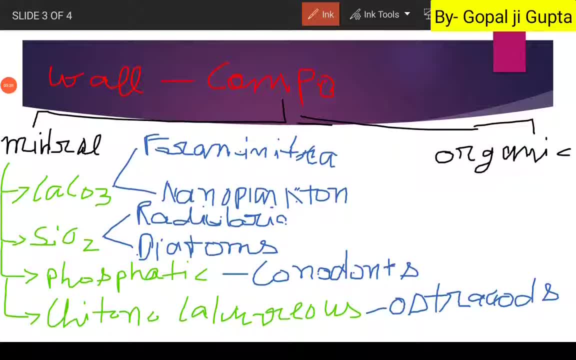 but the main, which are generally asked in many exams and you have to know these things. then we have the organic walled microfossils and the well-known two. first one is your dino flagellates. okay, d? i a n? o flagellates, okay. so this is the organic. 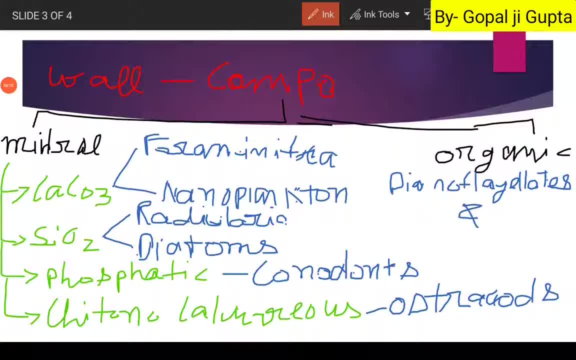 walled microfossil. and another one is, which is very known: is your pollen and spores okay, pollen and spores okay. so these are the general classification for the microfossils. so now let us summarize it. so we have classified on the basis of wall of composition. we have the mineral walled microfossils. 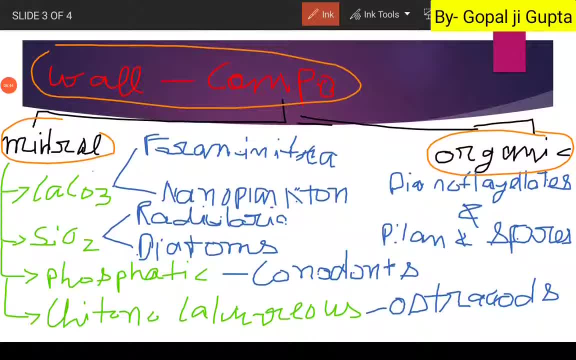 we have the organic walled microfossil. in the mineral wall we have the three type of minerals that are calcareous, siliceous, phosphatic and cytano calcareous. so in the calcareous wall we have the microfossils related to the micro sorry, related to the foraminifera. we